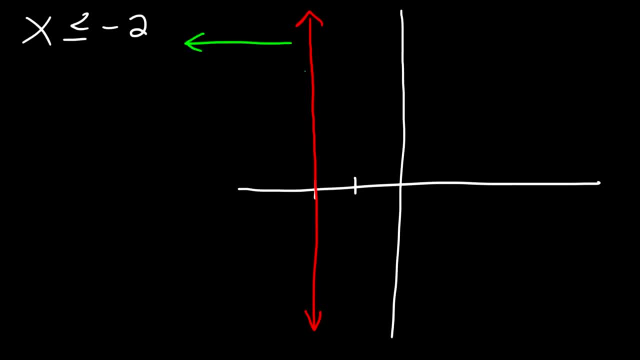 And less than is towards the left side. So the numbers that are less than 2 is going to be towards the left of 2. And so you have to shade everywhere to the left of this line. Now let's say if y is greater than negative 4.. 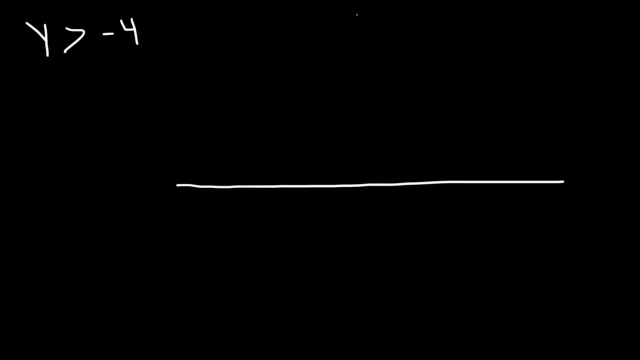 How can we graph it and where should we shade? So, whenever y is equal to a number, it's going to be a horizontal line as opposed to a vertical line, And because it's greater than, but not equal to, it's going to be a dashed line instead of a solid line. 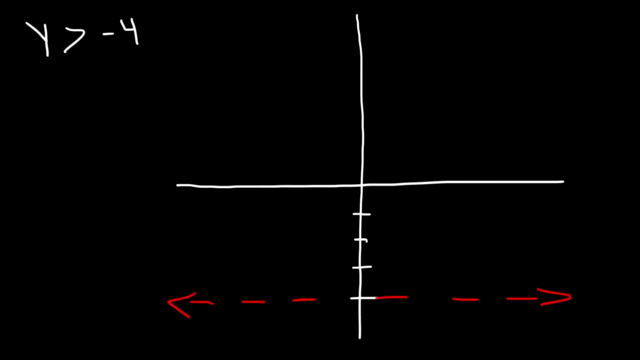 The numbers that are greater than negative 4 are above this line. So we need to shade in this region. And so that's it for this example. Try this one. Let's say if y is less than or equal to 2.. So this is going to be another horizontal line at 2.. 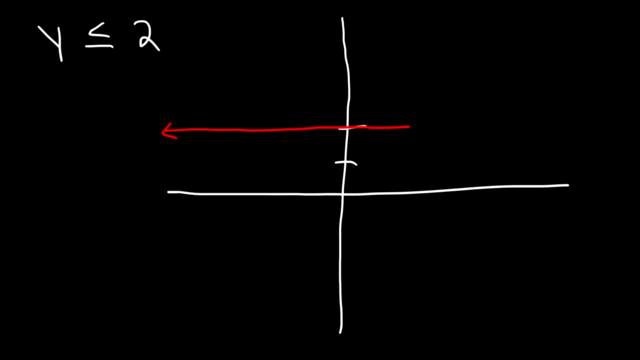 But because it's less than or equal to, it's a solid line as opposed to a dashed line, And because it's less than, we need to shade below it Rather than above, And so this is the answer. Now, what if we have an equation with two variables? 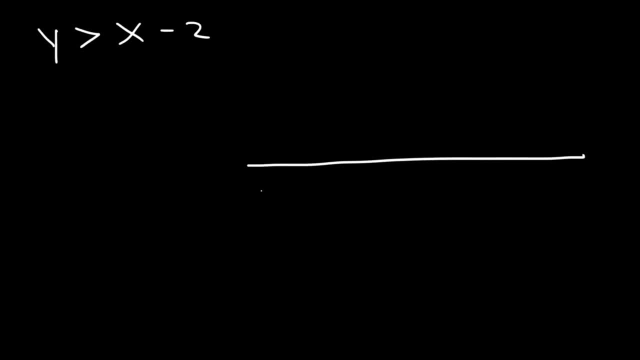 Let's say that y is greater than x minus 2.. How can we graph it? So this equation is in slope-intercept form. The number in front of x is the slope, So if there's no number, it's 1.. 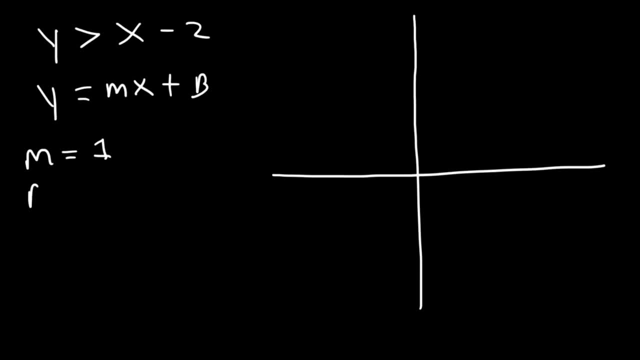 And the constant that you see on the outside, that's the y-intercept, Which is negative 2.. So the first thing you want to do is plot the y-intercept And then use the slope to find the next point. If the slope is 1, that means that rise over run is 1 over 1.. 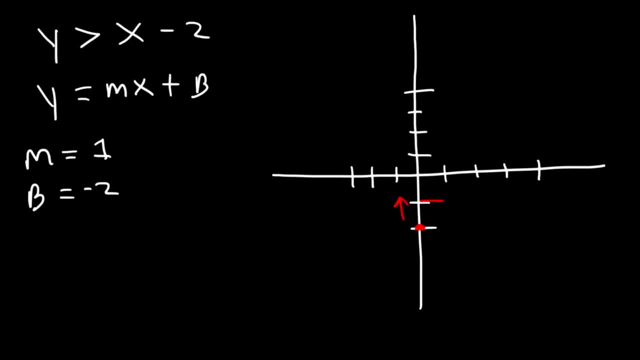 So as you go up 1, you need to travel 1 to the right. So up 1 is the rise, 1 to the right is the run. It's 1 over 1.. Because the slope is 1.. So therefore, the next point on the graph is here: 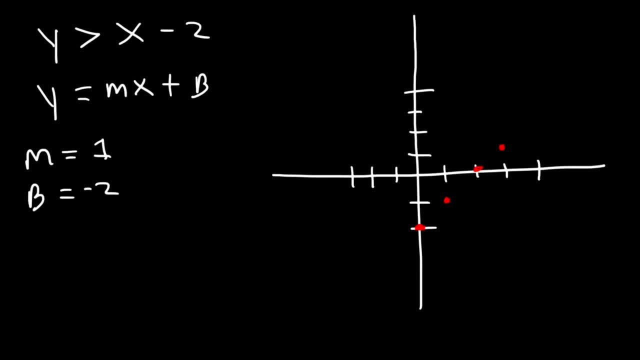 The next one will be here And here and so forth. Now it's greater than, but not equal to, So we're going to draw a dashed line through these points. Now notice that y is greater than the function, So we're going to shade above the line. 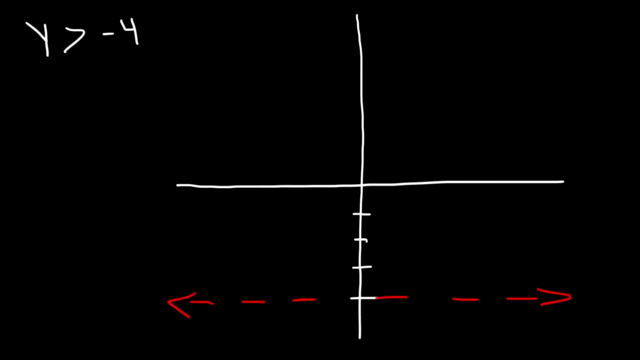 The numbers that are greater than negative 4 are above this line. So we need to shade in this region. And so that's it for this example. Try this one. Let's say if y is less than or equal to 2.. So this is going to be another horizontal line at 2.. 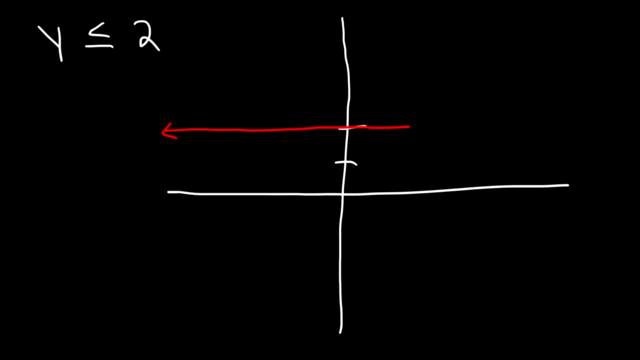 But because it's less than or equal to, it's a solid line as opposed to a dashed line, And because it's less than, we need to shade below it Rather than above, And so this is the answer. Now, what if we have an equation with two variables? 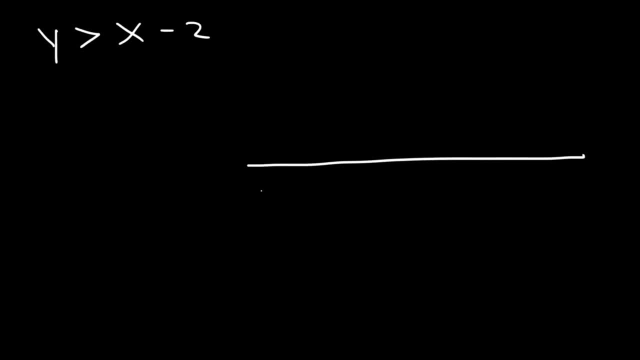 Let's say that y is greater than x minus 2.. How can we graph it? So this equation is in slope-intercept form. The number in front of x is the slope, So if there's no number, it's 1.. 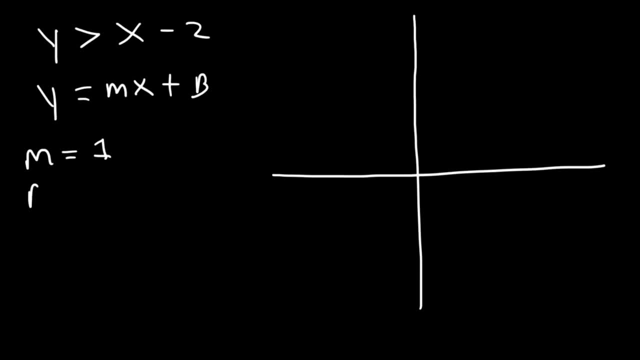 And the constant that you see on the outside, that's the y-intercept, Which is negative 2.. So the first thing you want to do is plot the y-intercept And then use the slope to find the next point. If the slope is 1, that means that rise over run is 1 over 1.. 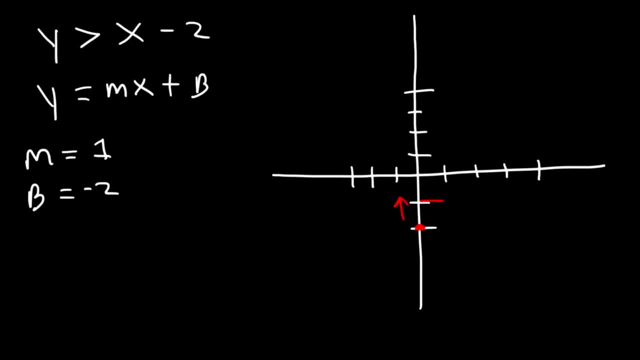 So as you go up 1, you need to travel 1 to the right. So up 1 is the rise, 1 to the right is the run. It's 1 over 1.. Because the slope is 1.. So therefore, the next point on the graph is here: 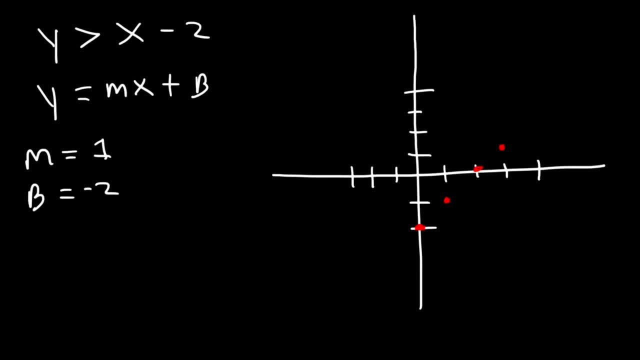 The next one will be here And here and so forth. Now it's greater than, but not equal to, So we're going to draw a dashed line through these points. Now notice that y is greater than the function, So we're going to shade above the line. 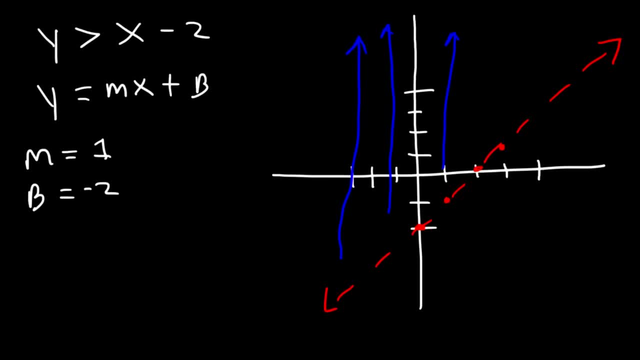 Rather than below it. So everywhere above it we're going to shade. And that's how you can graph it. Let's try one more example. Let's say y is less than or equal to 2x minus 3.. So we can see that the slope is 2.. 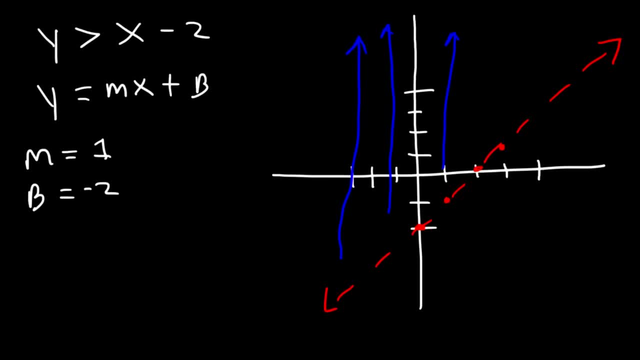 Rather than below it. So everywhere above it we're going to shade. And that's how you can graph it. Let's try one more example. Let's say y is less than or equal to 2x minus 3.. So we can see that the slope is 2.. 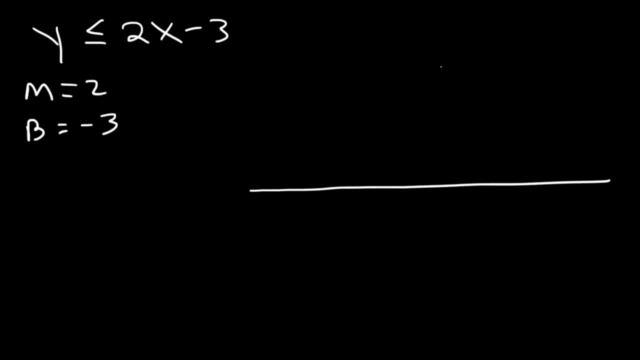 The y-intercept is negative 3. Let's go ahead and graph this function. So the y-intercept is negative, 3. And the slope is positive 2.. So let's start with negative 3. Now, because the slope is 2.. 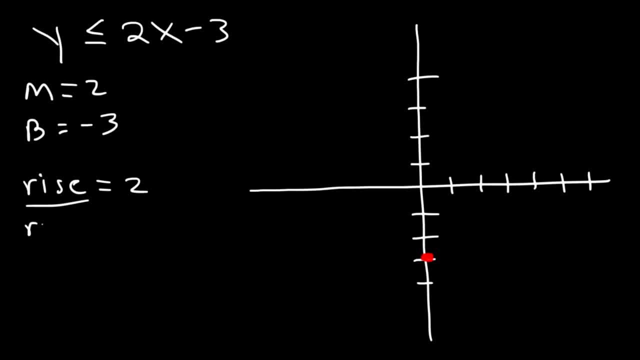 That means that the rise is 2. And the run is 1. Because 2 over 1 is 2.. So we need to go up 2 units because the rise is 2. And travel 1 unit to the right because the run is 1.. 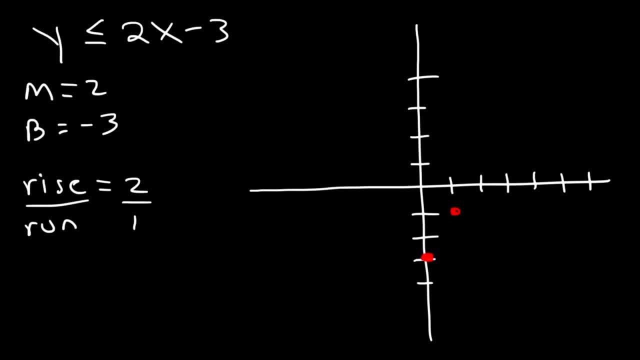 That will take us to the point 1.. And the slope is 2. Negative 1.. Then if we go up 2 over 1. That will take us to the point 2,1.. And then 3,4 and so forth. 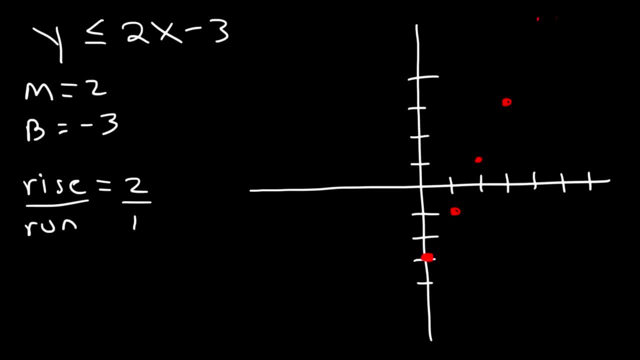 Now, because it's less than or equal to, It's going to be a solid line As opposed to a dashed line, And because it's less than the function, We need to shade In the region below it- Another way in which you can determine where to shade. 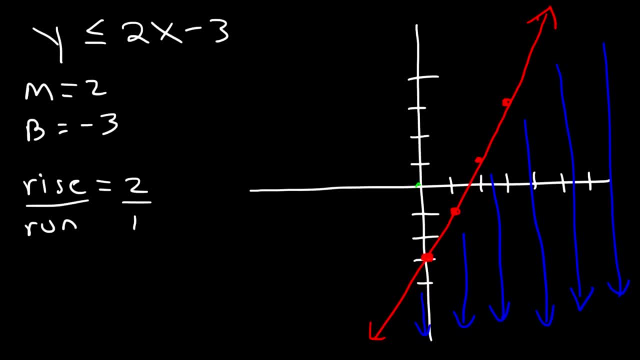 Is by using test points. Let's choose two test points, The first one being the origin, 0,0.. And another one, let's say, Let's choose this point, Which is 4, negative 2.. If the equation is true, then you should shade in that region. 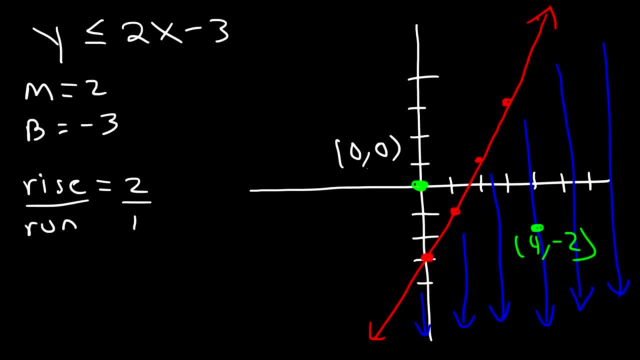 If it's not true, Do not shade it. So this should be Not true if we plug it in. So let's replace Y with 0 and X with 0. So 0 is less than 2 times 0 minus 3.. 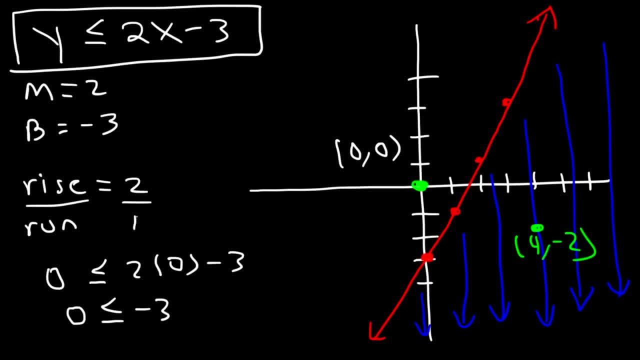 So is 0 less than negative 3?? On the number line it's not. 0 is to the right of negative 3.. And any number to the right Is greater than the numbers on the left. So this is not true. 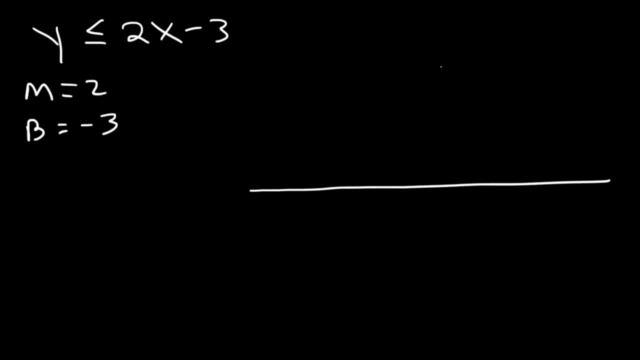 The y-intercept is negative 3. Let's go ahead and graph this function. So the y-intercept is negative, 3. And the slope is positive 2.. So let's start with negative 3. Now, because the slope is 2.. 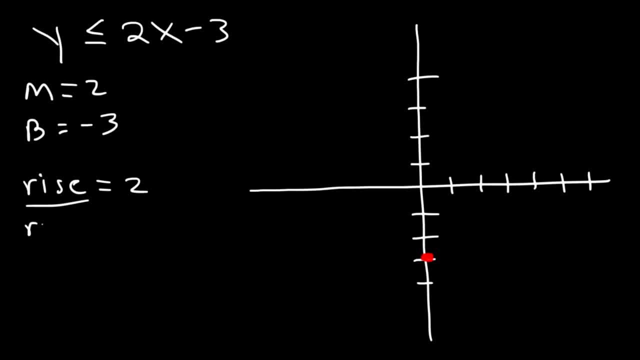 That means that the rise is 2. And the run is 1. Because 2 over 1 is 2.. So we need to go up 2 units because the rise is 2. And travel 1 unit to the right because the run is 1.. 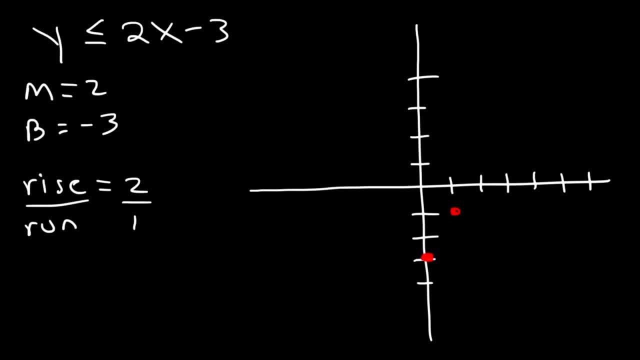 That will take us to the point 1.. And the slope is 2. Negative 1.. Then if we go up 2 over 1. That will take us to the point 2,1.. And then 3,4 and so forth. 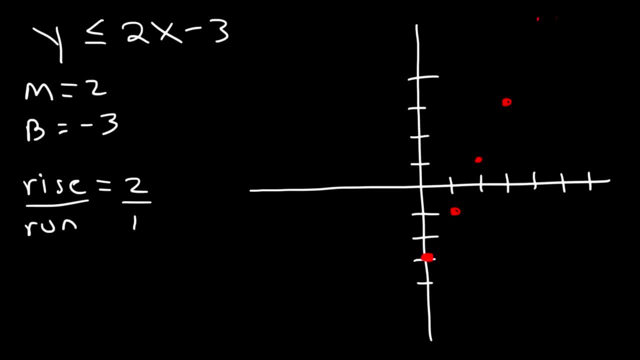 Now, because it's less than or equal to, It's going to be a solid line As opposed to a dashed line, And because it's less than the function, We need to shade In the region below it- Another way in which you can determine where to shade. 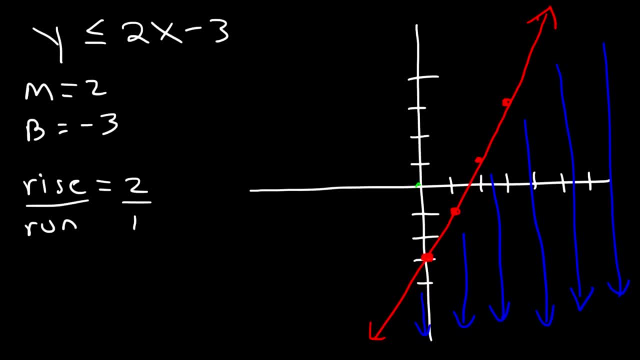 Is by using test points. Let's choose two test points, The first one being the origin, 0,0.. And another one, let's say, Let's choose this point, Which is 4, negative 2.. If the equation is true, then you should shade in that region. 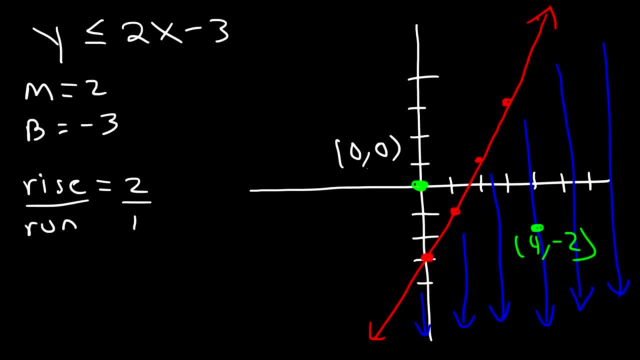 If it's not true, Do not shade it. So this should be Not true if we plug it in. So let's replace y with 0 and x with 0. So 0 is less than 2 times 0 minus 3.. 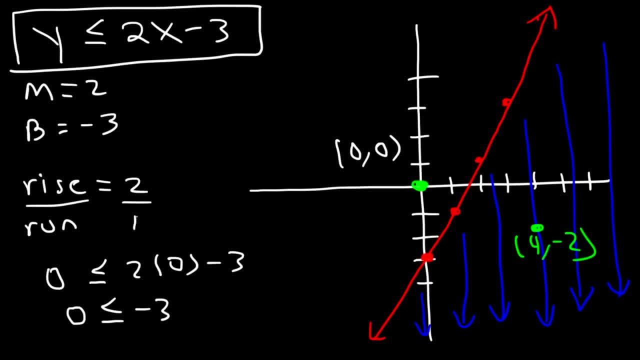 So is 0 less than negative 3?? On the number line it's not. 0 is to the right of negative 3.. And any number to the right Is greater than the numbers on the left. So this is not true. 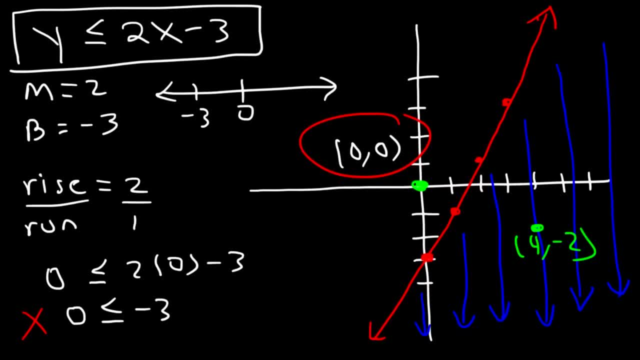 Which means that We should not shade in this region. Now let's test the point 4, negative 2.. Let's replace y with negative 2 and x with 4.. So 4 times 2 is 8.. 8 minus 3 is 5.. 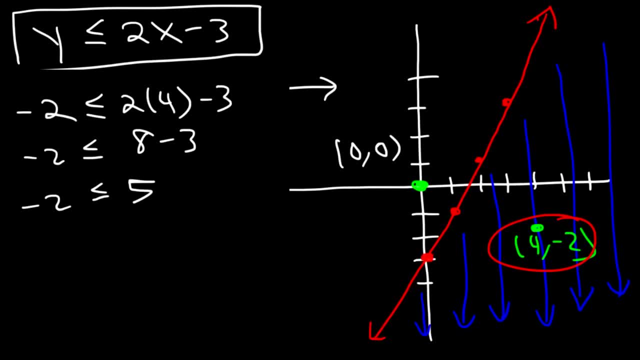 So is negative 2 less than or equal to 5?? Well, negative 2 is less than 5.. And if we read it the other way, 5 is greater than negative 2.. Both ways you read it, It's a true statement.